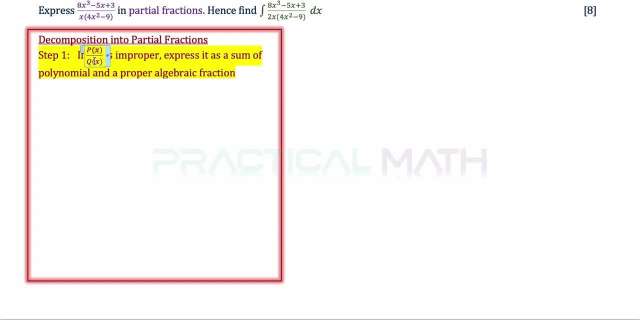 a degree that is greater than or equals to the degree of q of x, it is considered to be improper. we are to convert it to proper algebraic fractions by the means of a long division or a synthetic divisions or any other way, which i'll be showing you later on in this video. in step two, we have to: 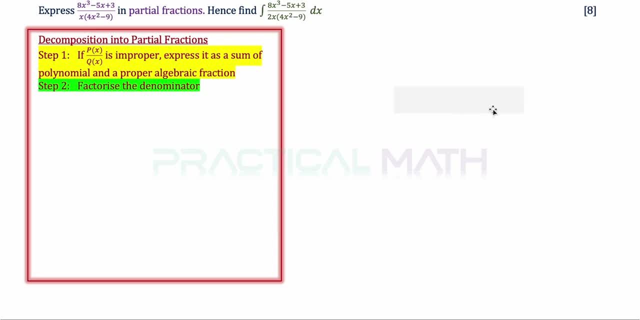 factorize the denominator. so before i go on to step three, let us first start off with our this part. one answer over here. so we are given these fractions and for us to use the alternative method, as mentioned earlier, i will have to expand the denominator out, in this case to give us a 4x. 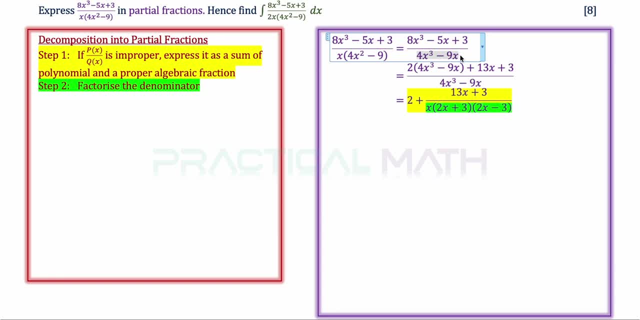 cubed minus 9x. so after expanding the denominator, we will take the highest term on top divided by the highest term below. so if we take 8x cubed divided by 4x cubed, it will actually give us a 2.. so to continue with this very 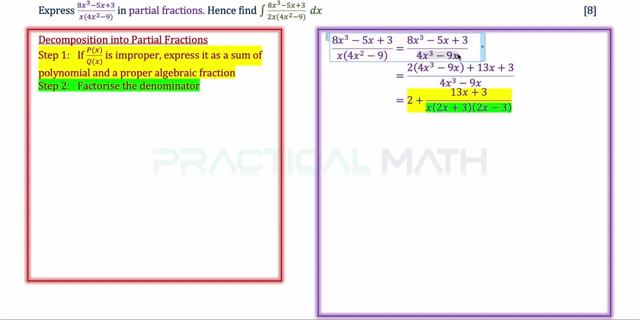 simple: we'll take 2 and we will multiply with the denominator of 4x cubed minus 9x. we close the brackets and we'll do a comparison between the numerator of both steps. so over here we take a 2 multiply by 4x cubed. i will actually have an 8x cubed in the previous. 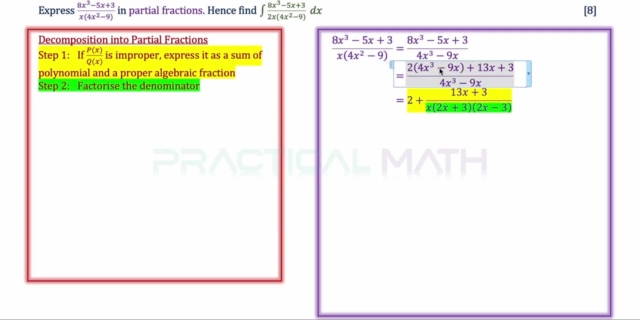 numerator. if i have a 2 multiply by a negative 9x, i will have a negative 18x. so negative 80x is not the same as the negative 5x. i'll have to plus an additional 13x, so negative 18x. 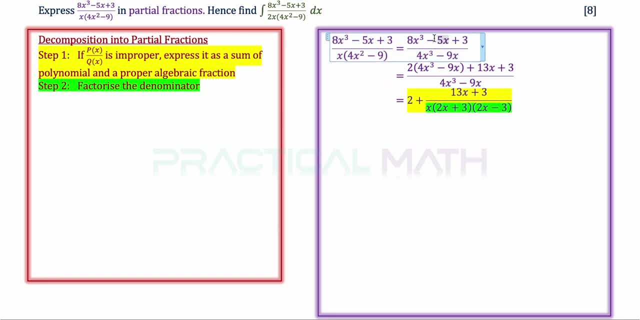 plus the 13x will now be the same as the previous step of negative 5x. the plus 3 is lacking, so i just put on a plus 3.. so in the next step we would have converted into a proper fractions. in this case, if i take 2 multiply by 4x, cubed minus 9x, divided by 4x cubed minus 9x, like this: 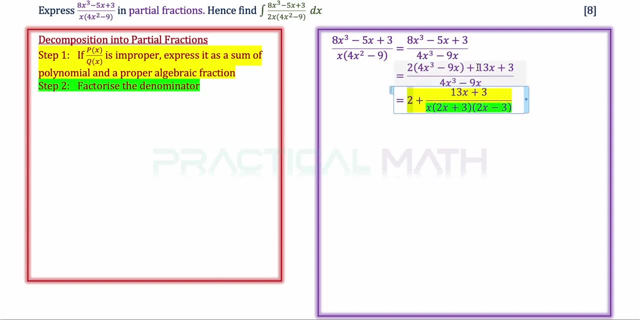 i will have the quotient of 2 and the remainder will be 30x plus 3 in the in the numerator like this and for the denominator parts i will be using this, but this is not the most factorized form, because we can use a special algebraic identity of a square minus b square to factorize. 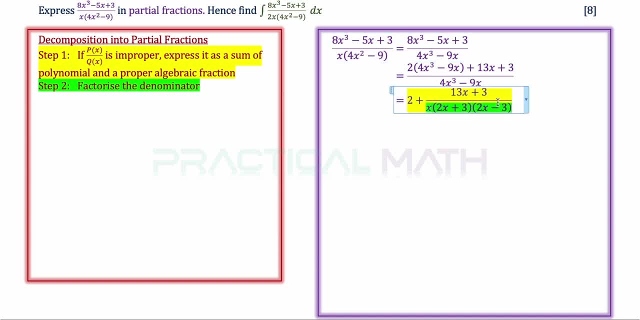 this into 2x plus 3 times 2x minus 3.. so, um, these three steps, um, there are many ways of doing it. the other way whereby we can use it slightly longer, you'll be using, through the long division, methods like this. so the step one is in yellow and the step two factorized. 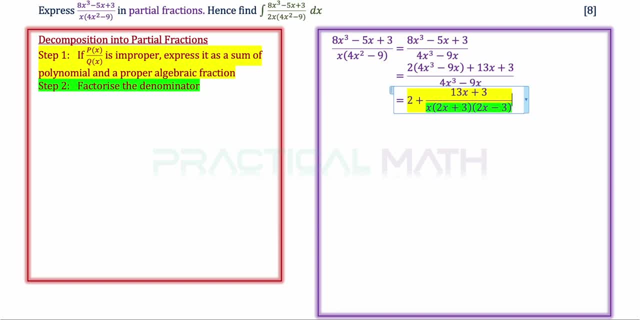 form will be in green like this. now, moving on to step three, let's go back to the left side, whereby we have to express it in the proper algebraic fractions in accordance to, uh, the next few steps. so case one: if it's a distinct linear factors, all right, if it's a distinct. 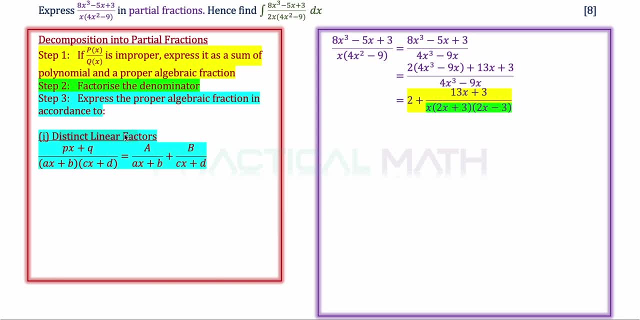 linear factors by distinct linear factors. we are referring to the linear factors at the denominator over here. now, as you can see that you have two linear factors of ax plus b and cs plus d because you have a power of one for the axis, and they are distinct because they are different from each. 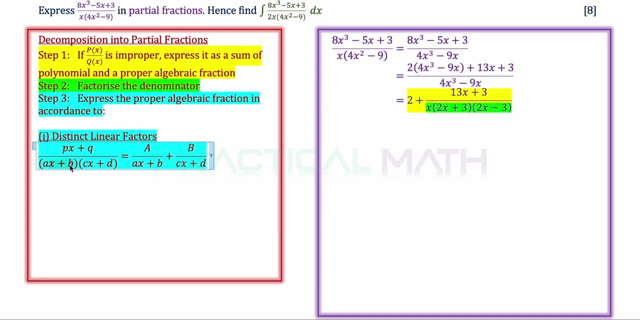 other. so this is the first linear factor, ax plus b. we express express it as a over ax plus b. for the second distinct linear factor of cs plus d, we express it as a b over cs plus d. for the second scenario, whereby, if your denominator consists of a repeated linear factors, 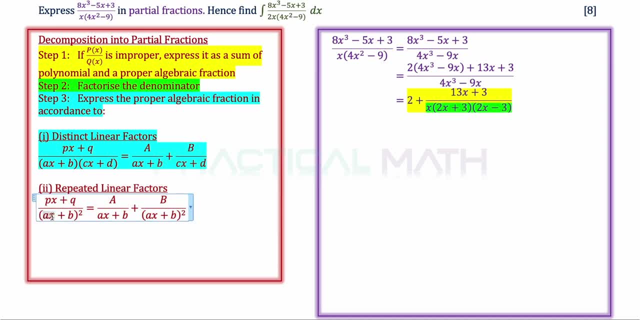 and, as you can see, for the denominator it is repeated because it's ax plus b, not power of one, the whole thing, power of two. then we'll use this b over ax plus b power of two, as well as a over ax plus b power of one. so, as you can see here it's ax plus b to the power of one and this is the ax. 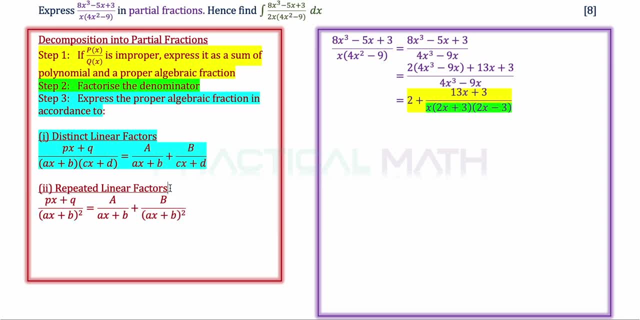 plus b to the power of two. like this, and moving on to the last parts, if your denominator consists of a quadratic factor of x square plus c square, where x square plus c square is in a numeric in the denominator and this cannot be factorized. so what i'm trying to say is x square plus c square refers to the factor that is in the 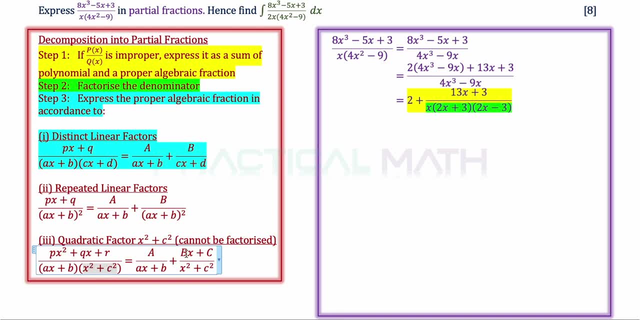 denominator and is quadratic, it cannot be factorized. we will use the formula of bx plus c over x square plus c square. now, as you can see here, the other factor is a linear ax plus b. we will still be using the distinct linear factor formula of a over ax plus b. now with these three, 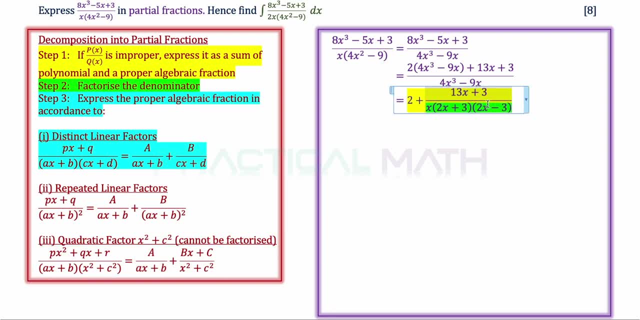 cases. we are to identify which of these three cases. it could be a combination of all three or now, as you can see, here we look for the denominator. you have an x, you have a 2x plus 3, you have a 2x minus 3.. there are three linear factors at the denominator, because they all have. 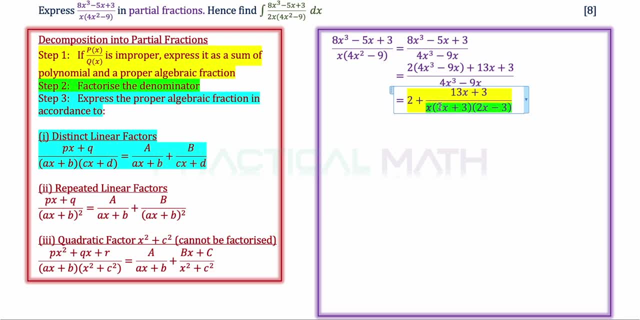 access to the power of ones and they are distinctively different from each other. so that means to say i'll be applying this blue color highlighted formula over here in our next step, so expressing as a proper partial fractions like this: um 13x plus 3 over this whole thing can. 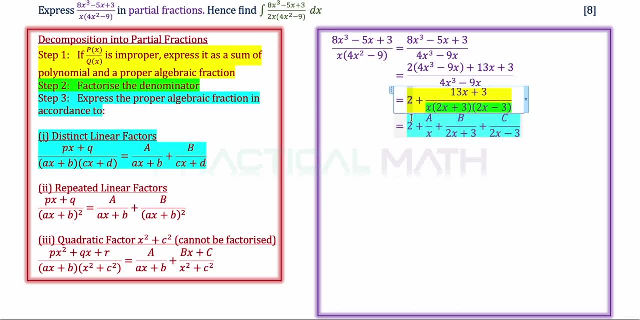 be used as a common denominator. so the next step is to express the non-linear factor of x. the fully linear factor will be the denominator, the number 3 and the linear factor of x and the denominator will still be the denominator of a over x and we will be expressing this as a. 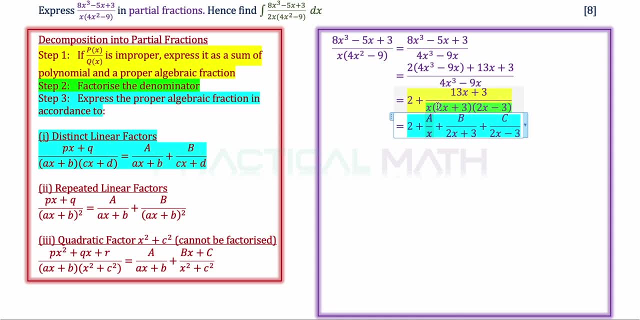 over x. we just want to be very clear about this part. take note that 2 must still remains, even though we may not need it for our next step, but it should still remain for it to be mathematically correct. so for the linear factor of x, in the denominator we express it as a over x. 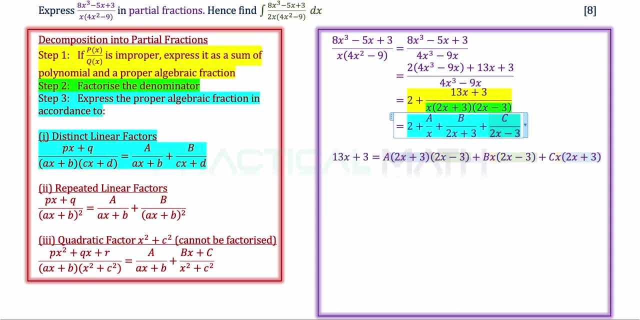 for the linear factor of 2x plus 3. in the denominator we express this b over 2s plus 3. step over here. what happens is we are going to convert this fraction, as well as this fractions, into a common denominator. what happens is that i'm going to express this as a common denominator of x. 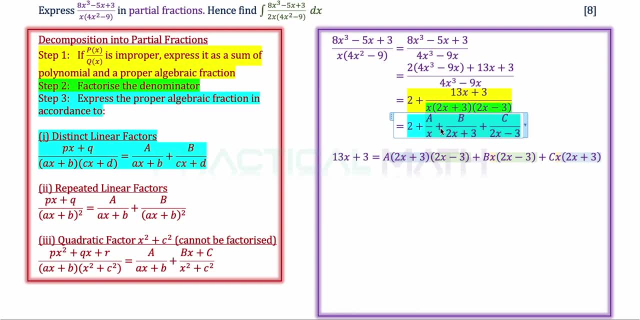 times 2x plus 3, times 2x minus 3. that means to say, for this part, here we will be lacking the denominator, will be lacking of a 2x plus 3 and 2x minus 3. so a must be multiplied by 2x plus 3 times. 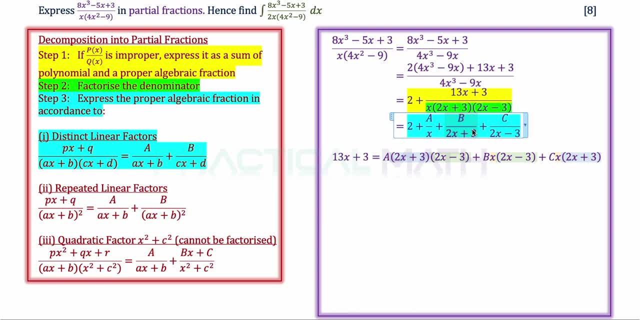 2x minus 3. for these fractions, the denominator, as we compare to the previous step, is lacking of an x and a 2x minus 3, so we multiply that to the numerator. for this fraction, the denominator is lacking of an x and a 2x plus 3, so we multiply it to the numerator like this, so comparing the 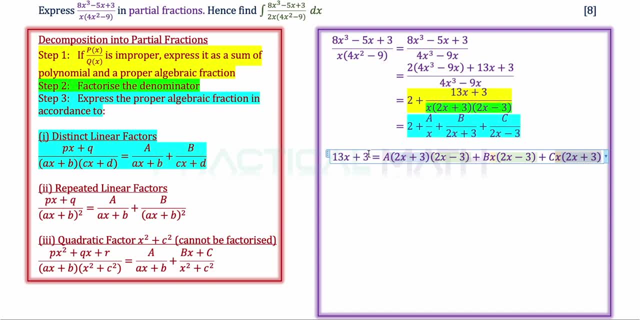 numerators of both steps, and the previous one is 13x plus 3. we have this polynomial identities like this. so, as you can see, here i did something whereby i highlighted the common brackets. you can see that this is a common denominator and this is a common denominator and this is a common 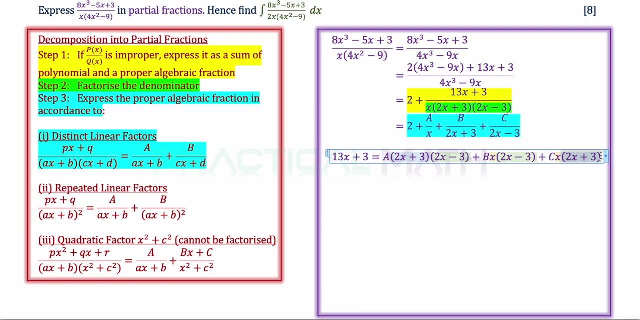 2x plus 3 is common, I highlighted in blue, And 2x minus 3 is common between these two terms. so I highlighted in green And I do have an x which is highlighted in orange for both terms, like this: 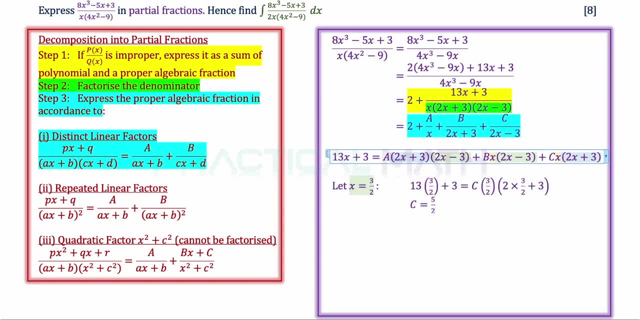 So in our next step we either do a comparing coefficients or substitution. Now for this question. I decide to use a substitution. Now what happens if I set this green to be equal to 0?? x will therefore be equal to 3 over 2.. 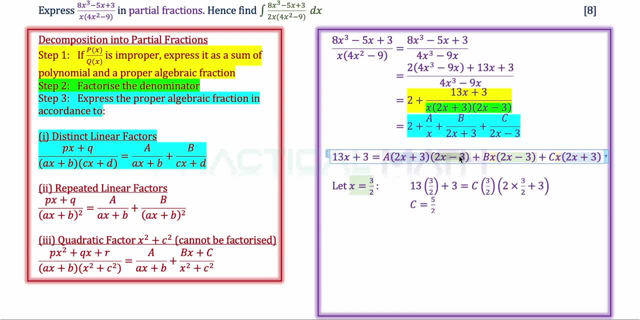 So if I set this green to be equal to 0, 0 multiplied by anything will be a 0.. So therefore, cancelling away this whole term, Because this green term has also been set to 0, 0 multiplied by anything will still be a 0.. 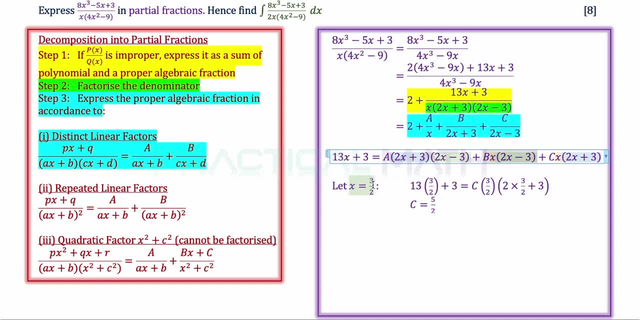 It will cancel away this whole term. Let's not forget that x is now set to be 3 over 2.. Replacing x to be 1.5 on the left: we will have this part on the left. Replacing x to be 1.5 on the right, it will be a c times 1.5, bracket, 2 times 1.5 plus 3.. 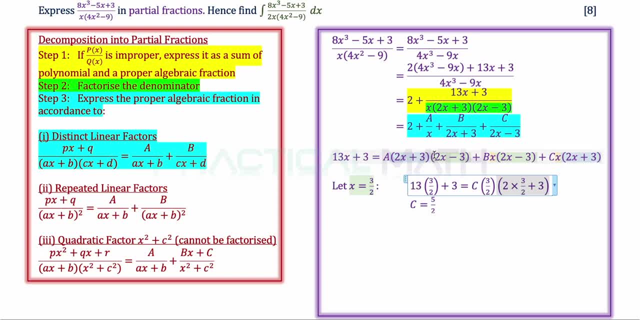 So, as you can see here, just by setting a green term, a green bracket, to be equal to 0, we can actually solve for c like this. Now, moving on to the next step, it's a similar fashion, whereby we set the blue now to be equal to 0. 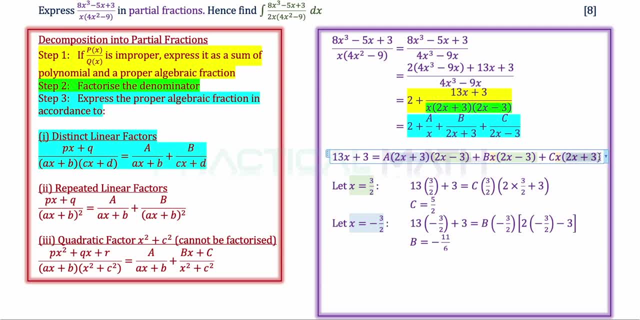 Set the blue term to be equal to 0. So we will have x to be a negative 1.5.. So if this is equal to 0, the whole thing here will be cancelled off, Because 0 multiplied by anything will be a 0.. 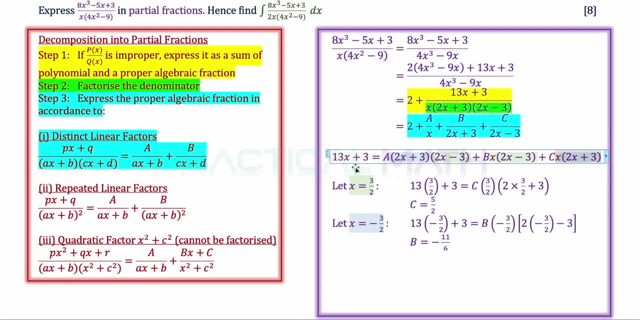 Likewise, this whole thing here will also be a 0. If I set x to be a negative 1.5, on my left I will be having this, And on my right I will have a b times a, 1.5 times this whole thing where I change the x to be a negative 1.5.. 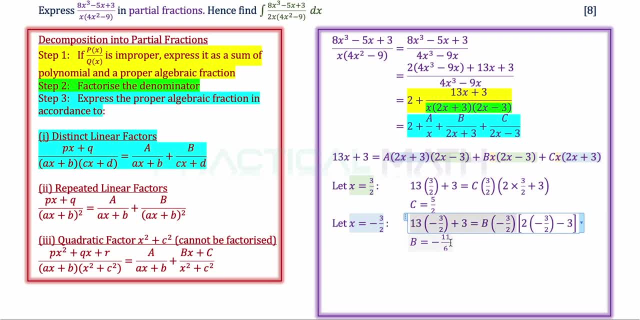 So solving for b from these equations, we will get this answer. Likewise, we can do the last part over here. If I let x to be a 0, which is the one that is highlighted in orange- If I let x to be a 0, this whole thing will now be 0. 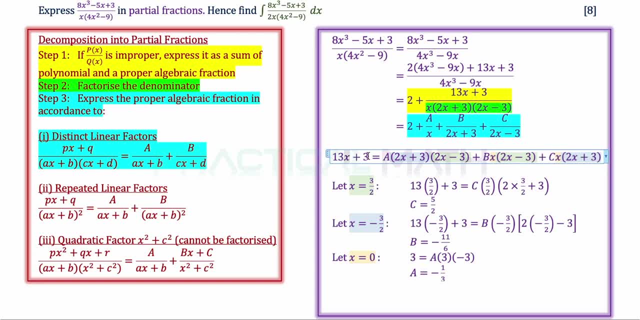 If I let x to be a 0, I will be left with a 3 on the left and on the right. I can just sub x to be a 0 to solve for a. So if a c to be a 5 over 2, b to be a negative 11 over 6, and a to be a negative 1.3,. 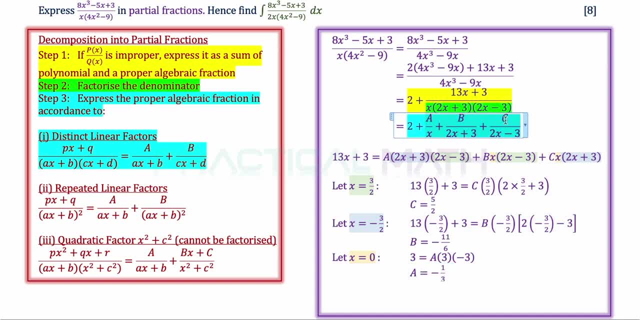 I will now want to replace into your a, b and c's in the previous step, like this to have this answer. So the proper partial fractions for the first part of this question will be 2.. Let's not forget we have a- 2 here. 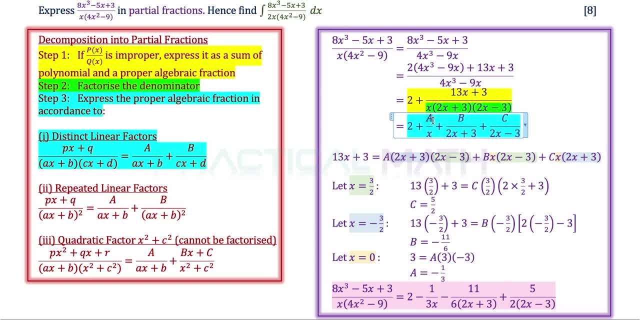 Since a is a negative 1.3, replacing a to be a negative 1.3, this fraction will therefore give us a negative 1 over 3x. Replacing b to be a negative 11 over 6, this fraction will now be a negative 11 over 6, bracket 2x plus 3.. 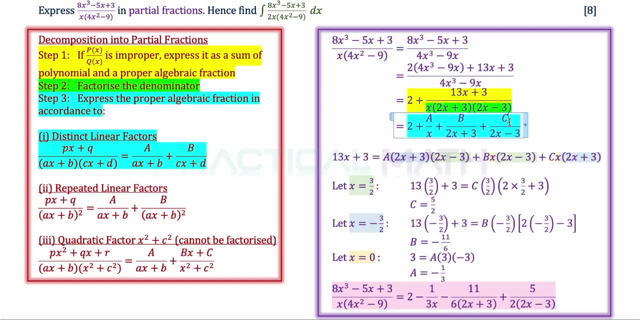 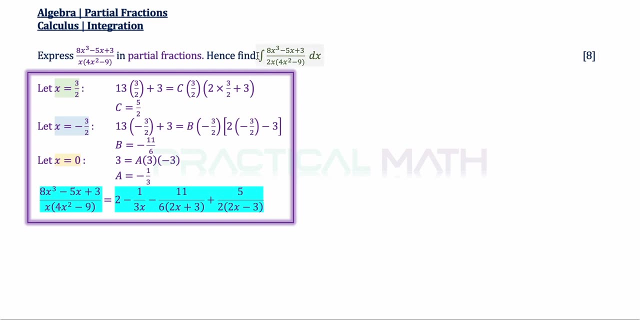 Replacing c to be a 5 over 2, this fraction will now be 5 divided by 2 times 2x minus 3.. And that's the answer for the first part of this question. For the last part of this question, we are told to find the integration of these algebraic fractions: dx. 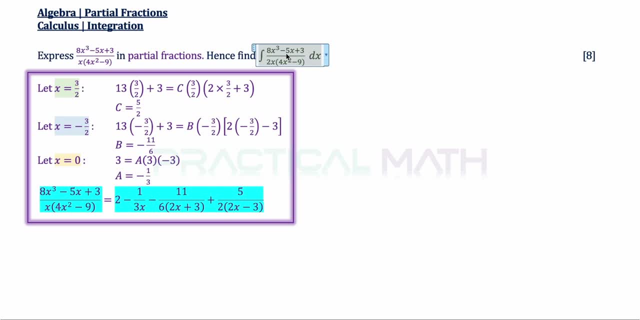 What I realized is that this is very similar to the previous parts, previous algebraic fractions we have done in partial fractions. So maybe for our first step let us first copy down this and identify what is common between both parts, like this: So over here, what is common between both parts I actually highlighted in blue: 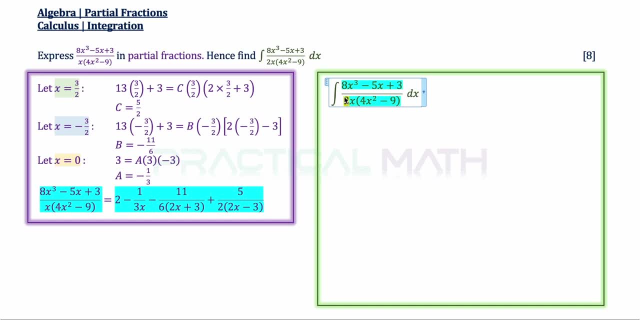 And what is different I actually highlighted in yellow. So, as you can see here, the common part is a 8x cubed minus 5x plus 3 divided by x, multiplied by 4x squared minus 9.. As seen in the previous parts, I put it on the left hand side of this presentation over here. 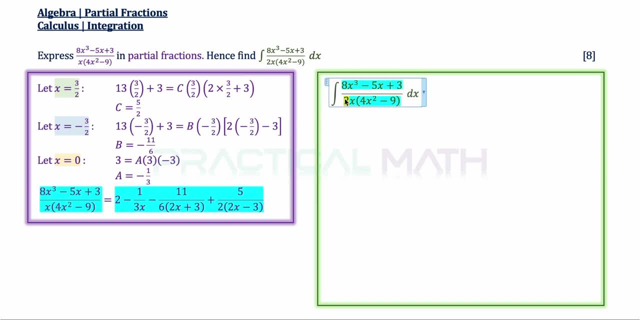 And what is different is just a 2 here. So in the next step I'm going to extract out this 2 in the denominator into a half. Alright, outside the integrations. So I'm able to do so because of the scalar multiplication rule of integrations. 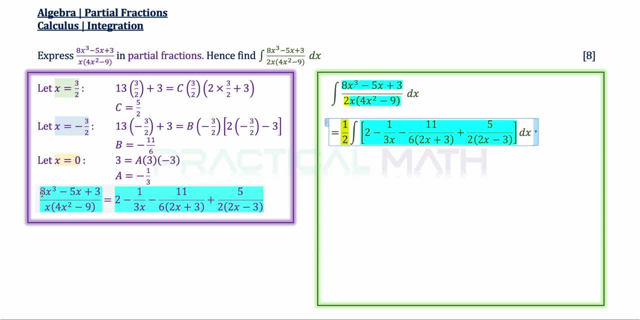 So I extract. I'm able to do so because of the scalar multiplication rule of integrations, So I extract it out, and what happens is that if I integrate the left, it should be the same as integrating the right. So, since we are integrating the left like this, alright, it should be the same as integrating the right side, like this. 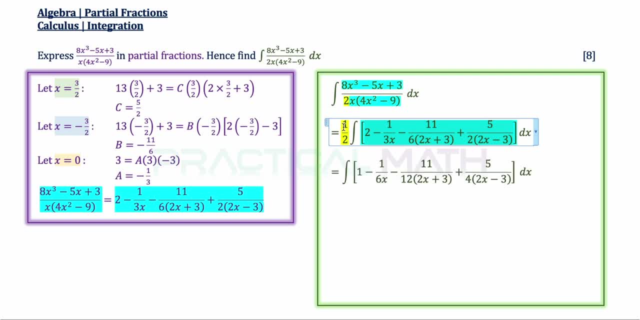 So in the next step I will be using the same rule, the scalar multiplication to multiplying the half. So half multiplied by 2 should give us a 1, and you do it for every individual terms. Half multiplied by a negative 1 over 3x should give us a negative 1 over 6x. 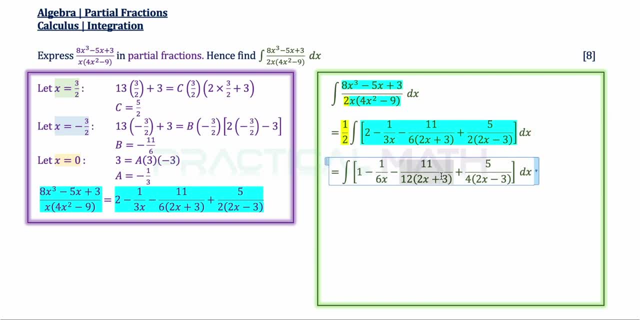 It should give us a negative 11 over 12 multiplied by 2x plus 3, and you do it for the last term as well. So over here we have an integration of a series of terms. I don't like to be in such a way. 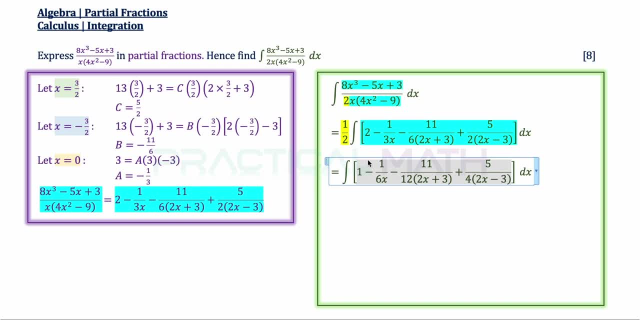 It looks very complicated because you have difference of terms inside. I want to split it into integrations of separate terms like this. So basically, integrate 1 dx minus the way integrates of these parts here. So over here let's look at the difference between this and this is that I took out the constants of 1 over 6 on our sides. 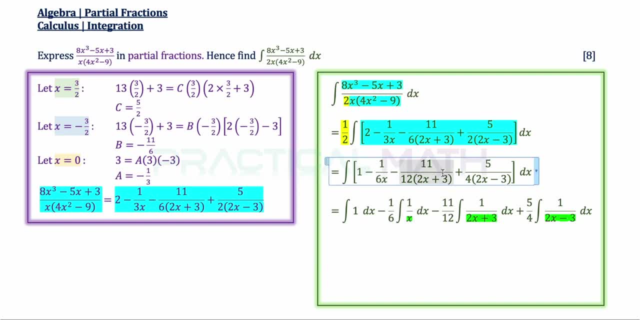 I'll be left with integrate 1 over x. Likewise, for this part, let's look at. the difference is that I take out the constant once again of 11 over 12: integrates 1 over 2x plus 3.. And over here I took out the constants of 5 over 4: integrates 1 over 2x minus 3.. 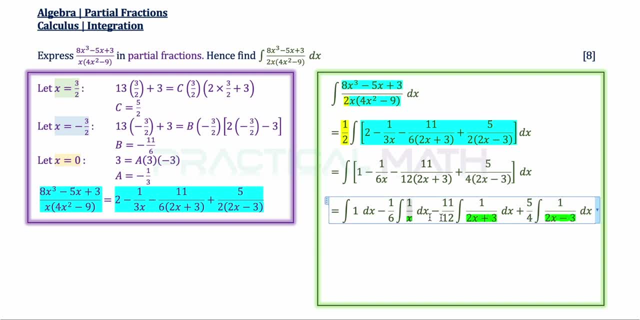 Now we have something in common between the last three integrations: 1 over x, 1 over 2x plus 3.. 1 over 2x minus 3 dx. That is the integration of the form of 1 over ax plus b dx. 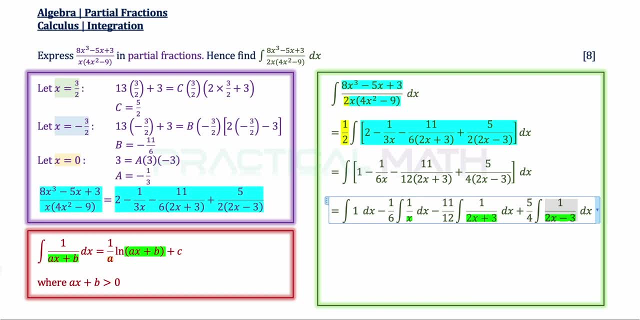 So I'm going to show you the next formula like this: on the left side, If you are to integrate 1 over ax plus b, dx, the result will actually give us 1 over a ln, ax plus b plus c. So this is one of the rules of integration that we have, one of the integration techniques. 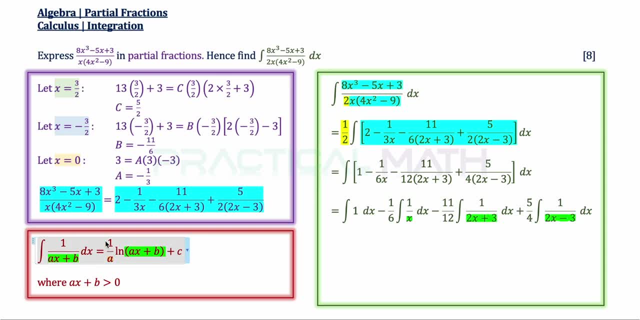 So if I integrate 1 over ax plus b dx, it should give us 1 over a multiplied by ln, ax plus b dx. So 1 over ax plus b, dx plus c, where c refers to the arbitrary constants and ax plus b must be greater than 0, because we cannot ln a 0 or ln a negative. 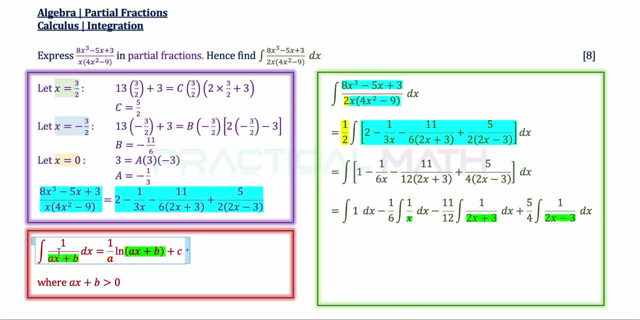 It must be greater than 0.. So over here, as you can see, I highlighted in green. So the fractions will go into the ln part And you're going to divide by the differentiation result of your denominator. So 1 over a refers to the differentiation result of the denominator. 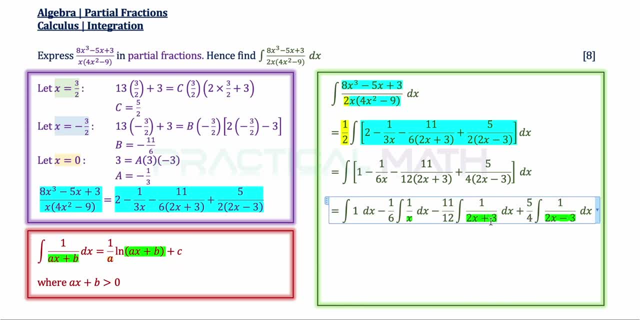 And you divide it like this. So I've highlighted in green: We're going to take ln to all of this in our next steps. So over here, integrate x is actually a 1x. Integrate 1 is actually a 1x, like this: 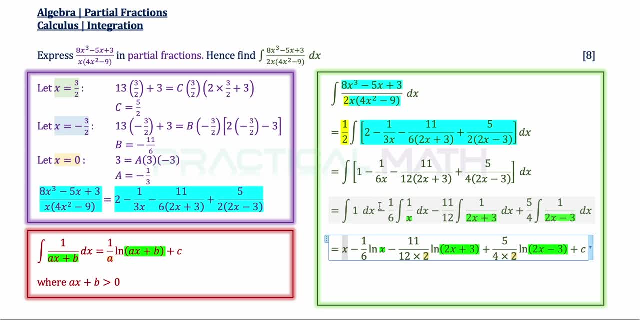 And integrate a negative 1 over 6 multiplied by 1 over x. Now 1 over 6 will remain. Don't worry, because it's a scalar multiplication. Integrate 1 over x is just simply ln x. Now integrate 1 over 2x plus 3.. 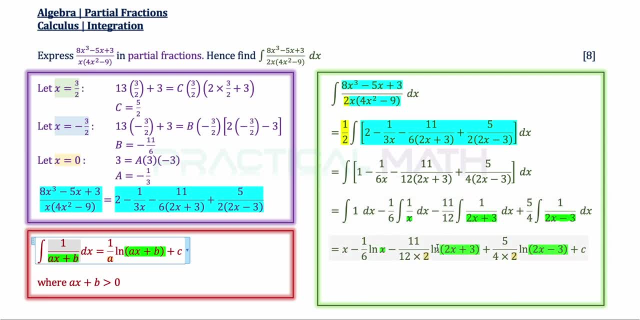 In this form. like this, we will have a ln 2x plus 3. That's for sure- Divided by the differentiation result of the denominator. The differentiation result of the denominator in this case is a 2. So I have to divide by 2.. 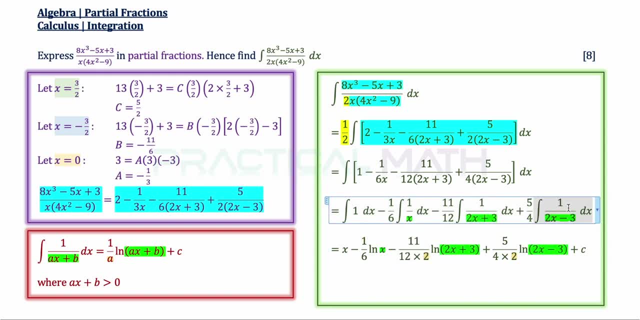 As you can see, I highlighted in orange. Likewise, if I'm to integrate this, I will have a ln of 2x minus 3 written in this form, divided by the differentiation result of the denominator. In this case it's another 2.. 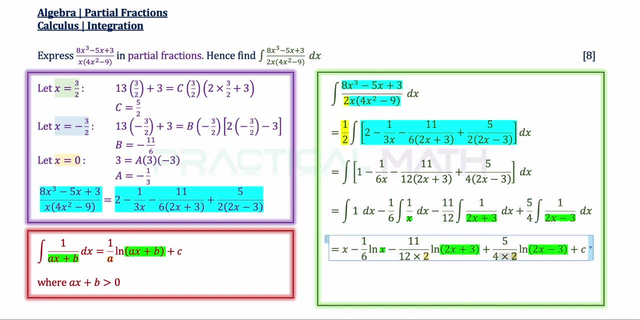 Multiplied by 2 to the denominator, like this, So simplifying in the next part, will give us this answer over here. So 11 divided by 12 times 2 is 11 over 24.. 5 divided by 4 times 2 will give us 5 over 8.. 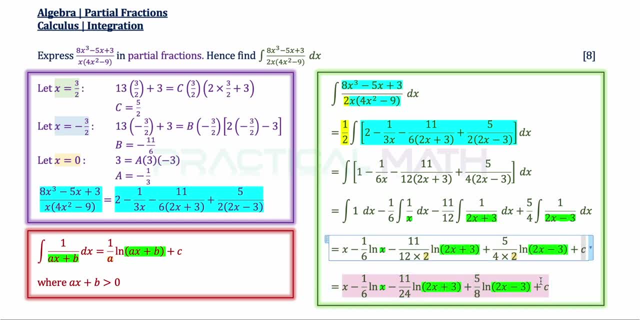 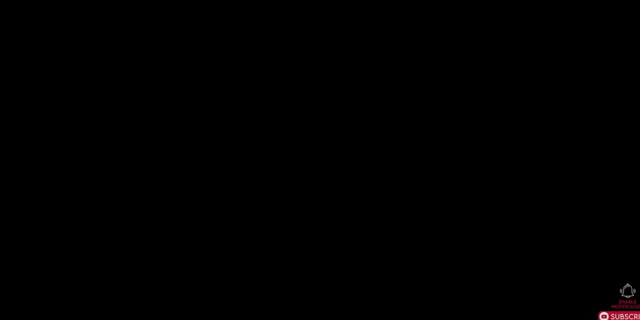 Let's not forget to put in all the arbitrary constants of C. So with this, that's the answer for this whole question. Alright, thank you for watching. I hope you have learned something again And see you in the next question. Thank you.